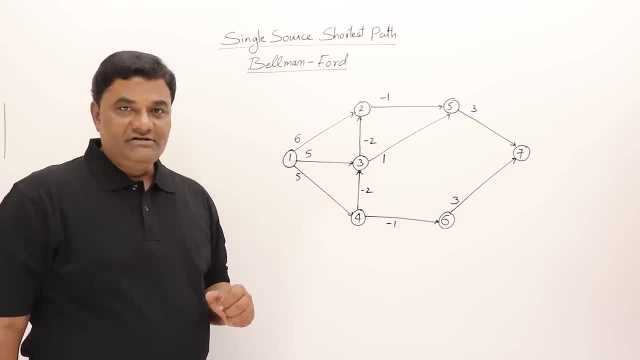 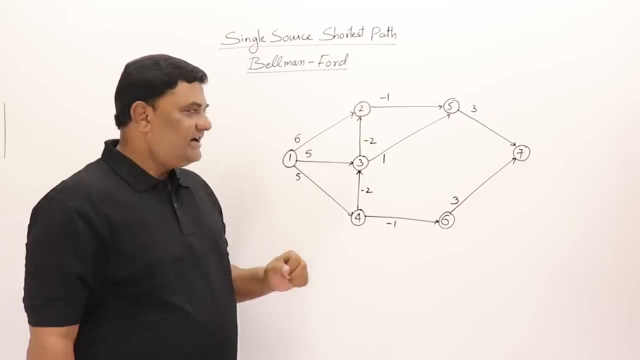 and it follows dynamic programming strategy. So dynamic programming strategy says that you try out all possible solutions and pick up the best solution. So here we want to try out all possible solutions and pick up the best solution, How we will try all of them. So this algorithm says that you go on relaxing all. 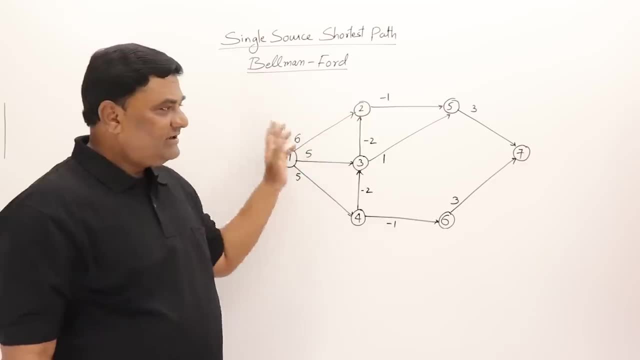 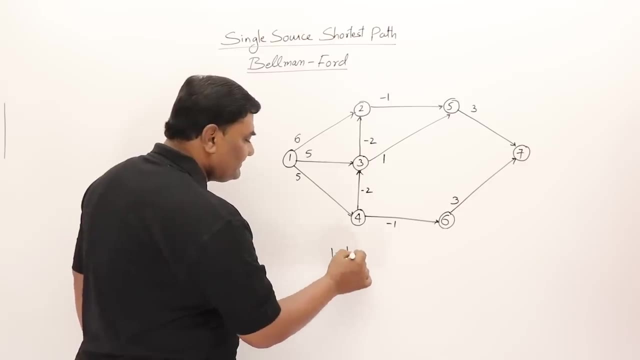 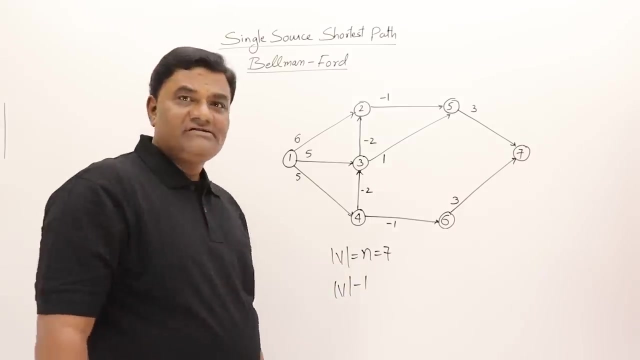 the edges. How many times? All edges. you repeatedly relax them for n minus one time. What is n here? n is the number of vertices. Number of vertices are 7. So I should relax them for 7 minus 1.. What is the idea here? If from the source vertex, if the 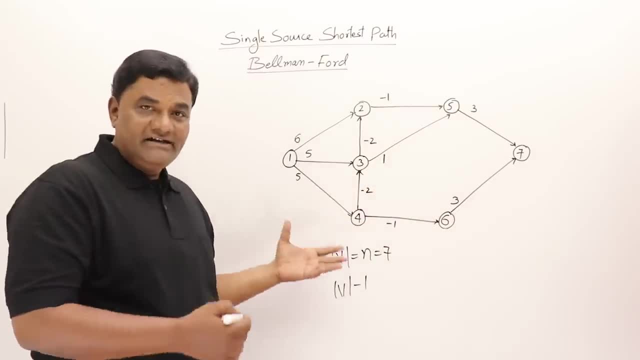 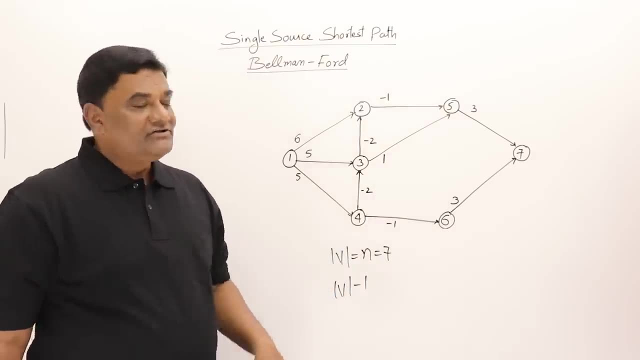 longest distance may be of all edges, then total how many edges may be there. So from 1 to 7, there can be maximum 6 edges. So if you are going on relaxing the edges we may get a longest path also. that is of 6 edges, So it will cover all possible paths if you relax all of them. 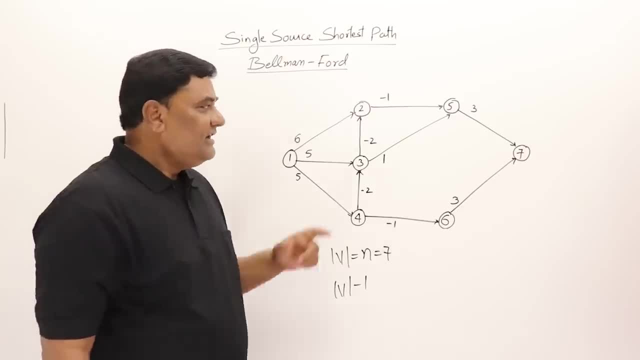 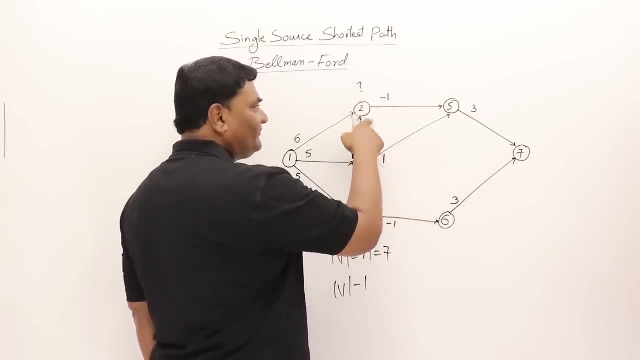 For 6 times. So what is relaxation? If I take any two vertices, let us say 2 and 5, and I know some distance of this vertex, the path to this vertex and the path to this vertex also, then I should see that if the path of this one plus this is less than this one, If so, I will change this. 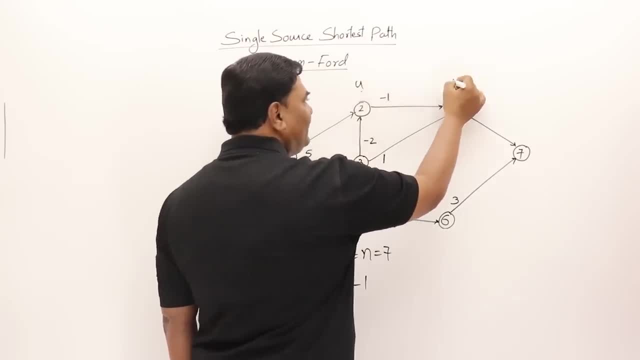 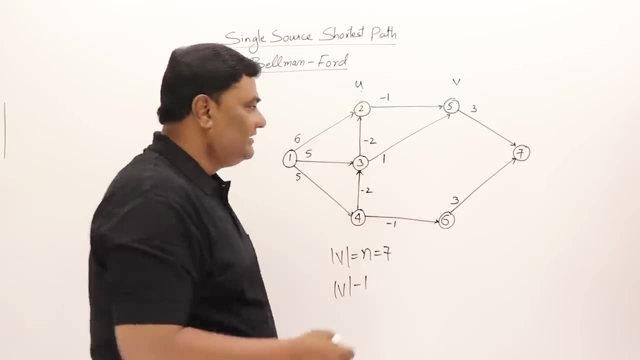 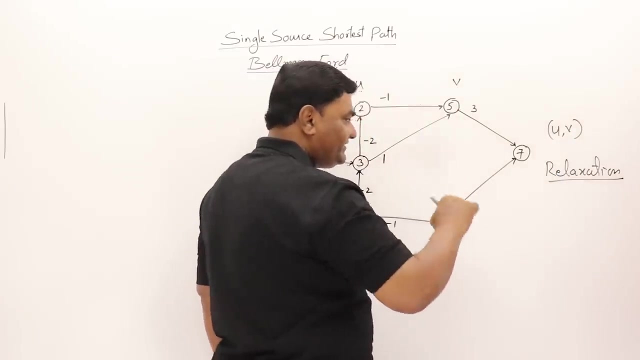 one. So I will call them as u and v and I will write down- just I will write down- what does relaxation mean. So then, once I, once I start using it, I can explain you how it works. So relaxation means what Between a pair of vertices u comma v. if there is an edge, then check if the distance of u plus. 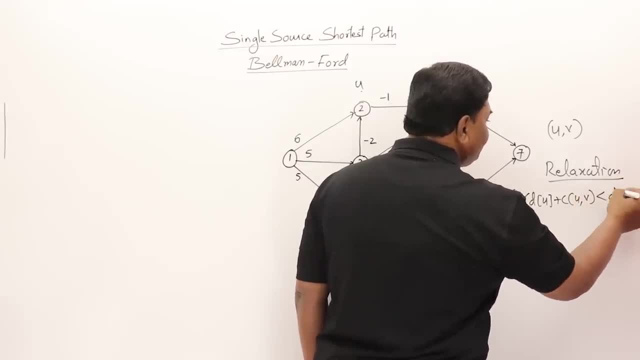 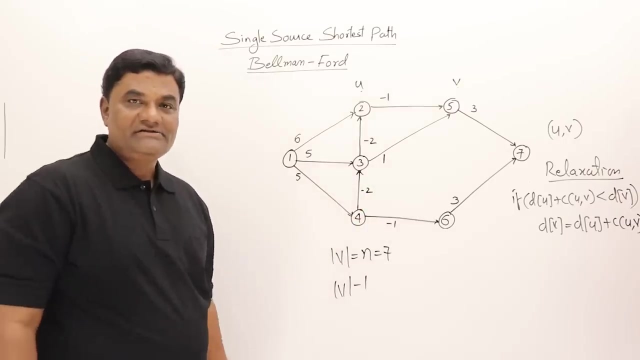 cost of an edge u comma v is less than distance of v. If so, then change the distance of vertex v to distance of u plus cost of an edge u comma v. What is that? I will explain you while solving this. Now let us follow the algorithm. What the algorithm says, you prepare. 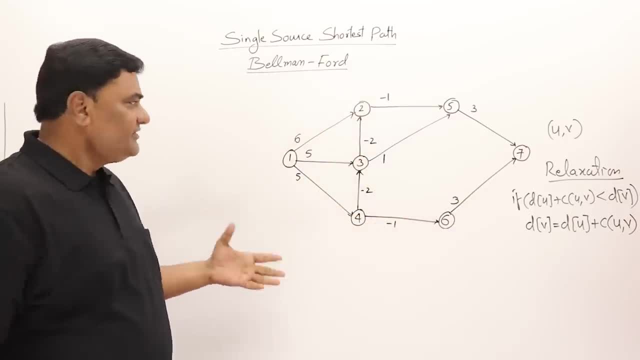 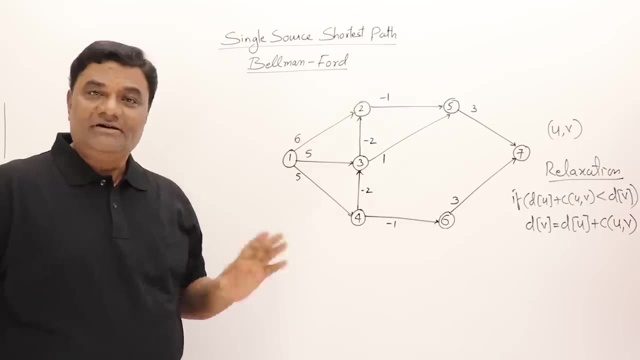 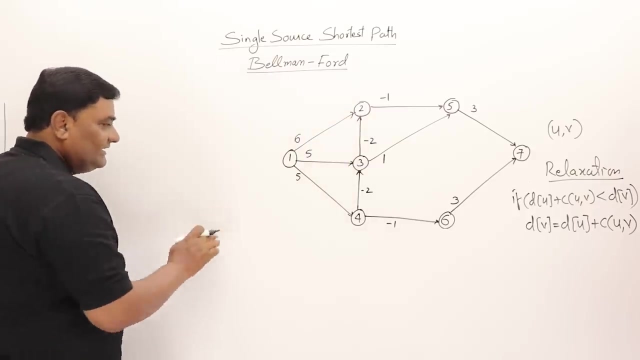 the list of all edges, Prepare a list. So which edge I should select first. You select any edge. first you select this one, then this one, or this one or this one. you select anything, but make sure that all edges are selected. So I will select them vertex by vertex. So I will write down the. 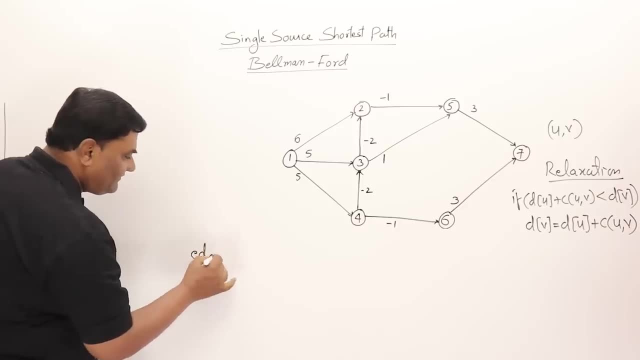 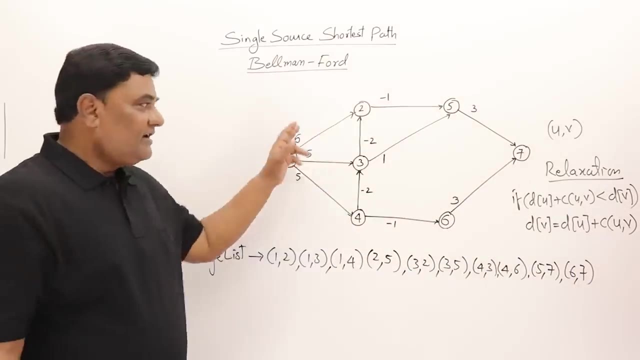 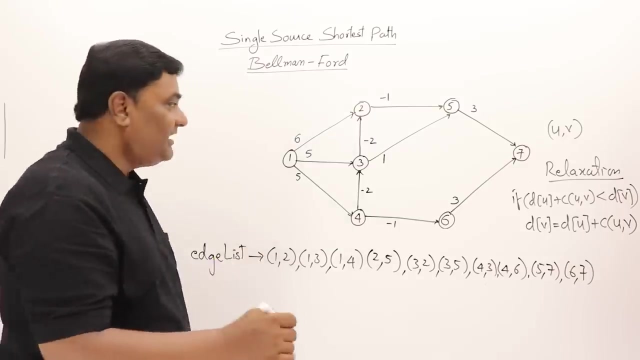 list of edges. here There are total 10 edges. I have taken all 10 edges here. List of edges. Now I have to relax all these edges for six times. Now let us start the procedure For that. initially, I have to mark: 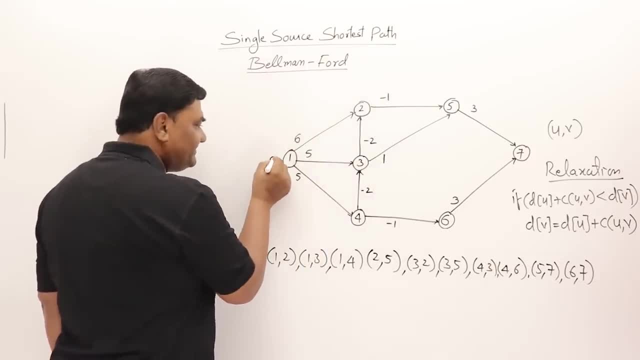 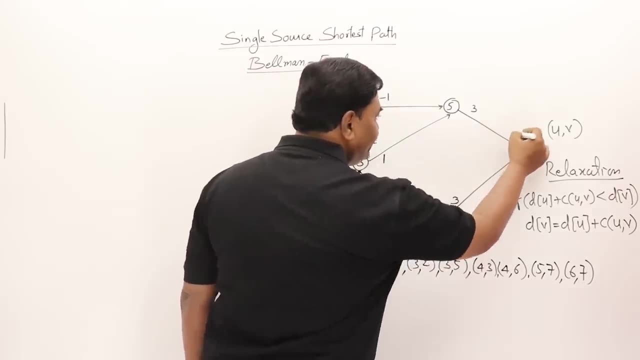 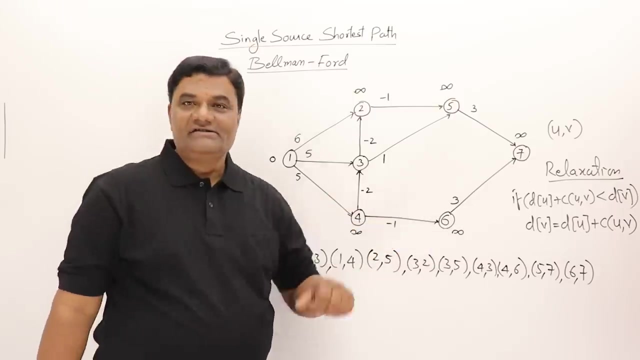 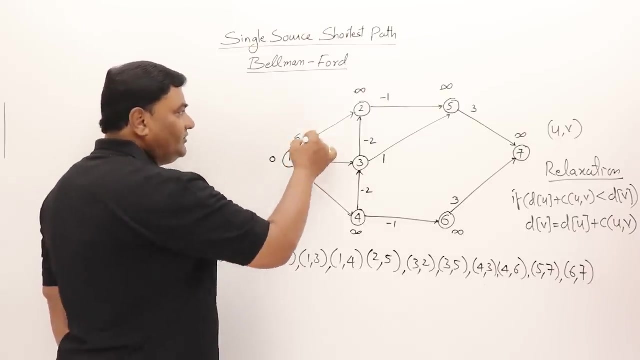 the distances of all these vertices. So this vertex, let it be zero. and for all other vertices, mark the distance as infinity. Mark it as infinity. All are infinity. Now start relaxing the edges. Now I will show you how that relaxation procedure works. First edge: 1, comma 2, 1 to 2.. What is the distance of this one? Zero? What is the distance? 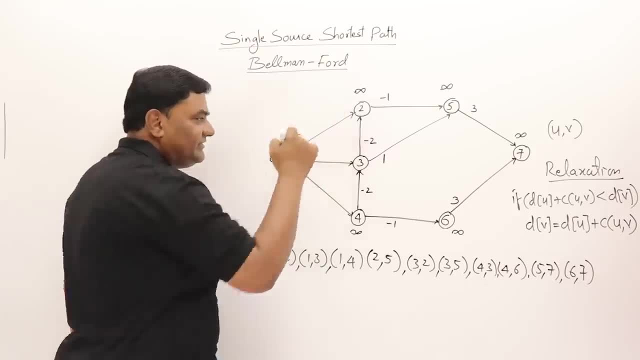 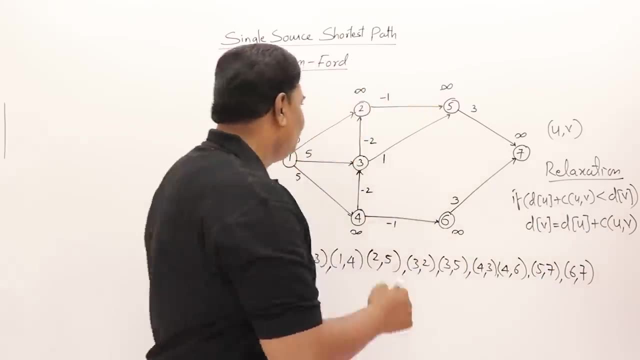 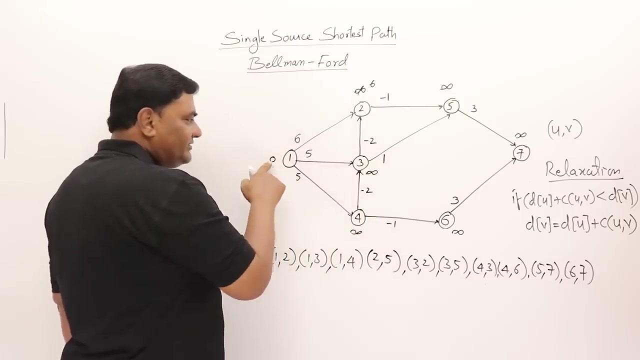 of this infinity. Zero plus six is less than infinity. Zero plus six is less than infinity. So change this infinity to zero plus six. So make it as six. The next one comma, three, zero, and this is infinity. So zero plus five is less than infinity. So change this to five. 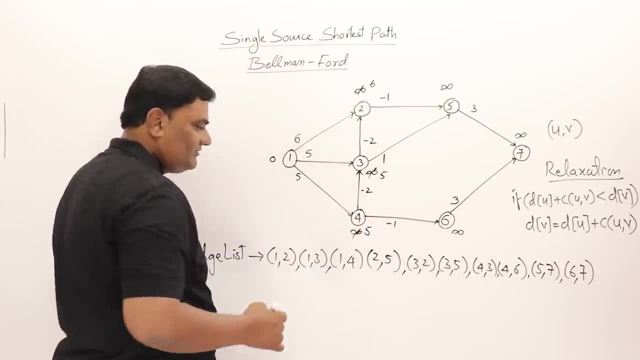 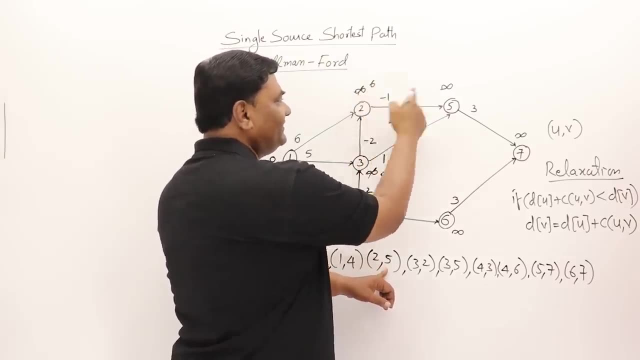 Zero plus five is less than infinity, So change it to five. So first three edges completed, Now two comma five. Two comma five. This is six minus one. This is infinity. So this is five. Six minus one is five. This is already changed, You see. 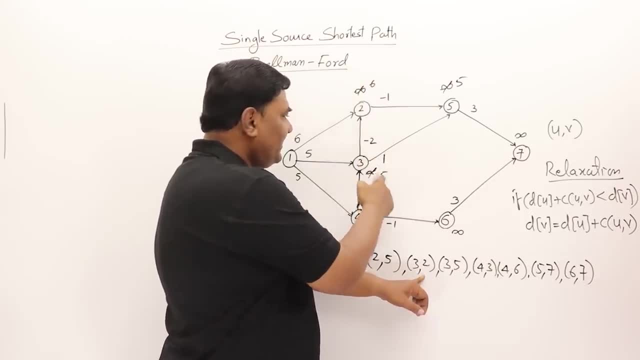 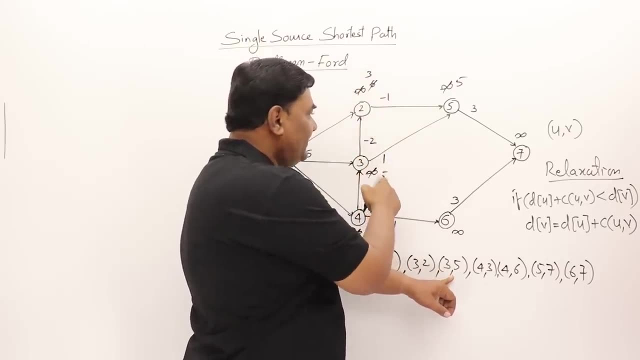 Three comma two, So three to two, So this is five minus two is a three, So change it to 3, then 3 to 5, so this is 5 plus 1 is a 6 and it is 5, so that is smaller, don't modify. 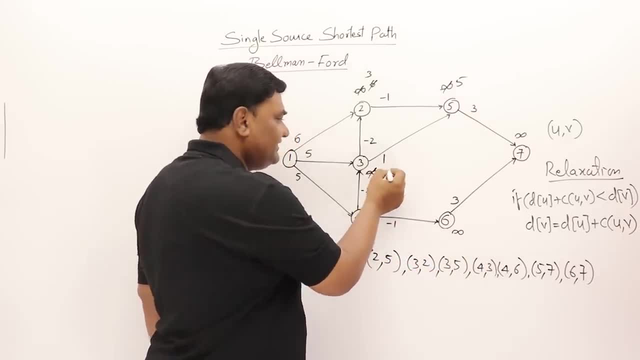 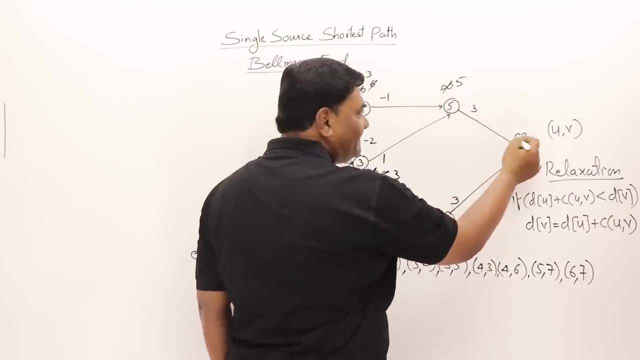 that one 4 comma 3, 5 minus 2 is a 3, so this becomes 3. then 4 comma 6: 5 minus 1, this is 4. this is infinity. so change it to 4. then 5 comma 7, so 5 plus 3 is 8. this is infinity, so change it to. 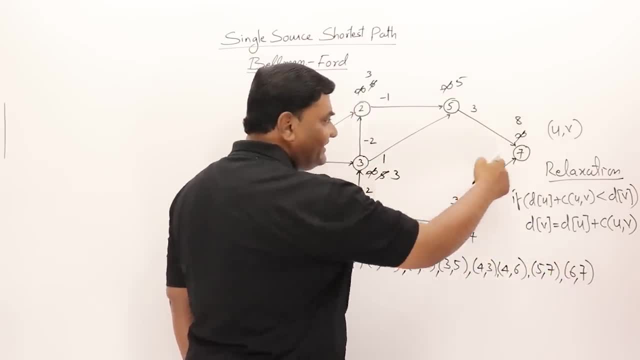 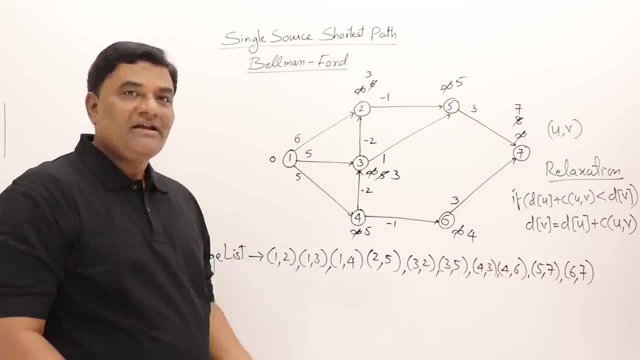 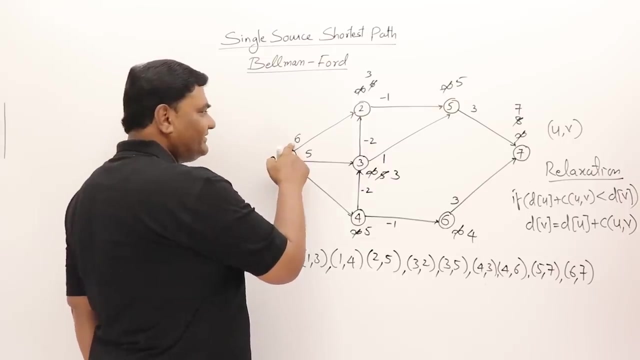 8, 6 comma 7, 4 plus 3 is 7. this is less so change. so most of the changes we have seen first time only let us continue second time. 1 comma 2, so 0 plus 6, 6 and 3, so this is greater than that one. 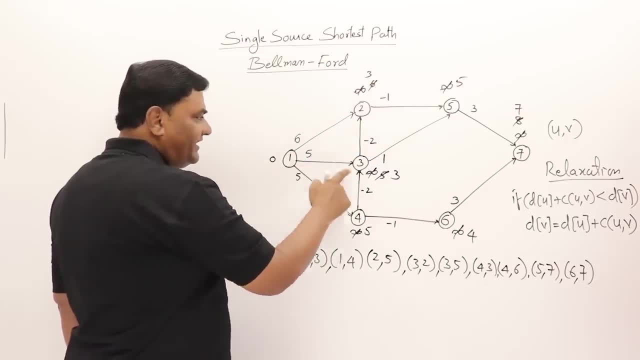 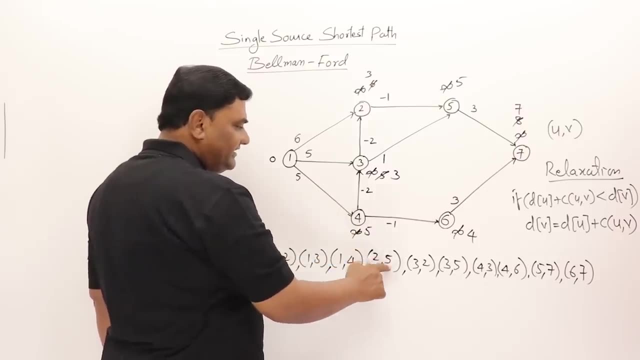 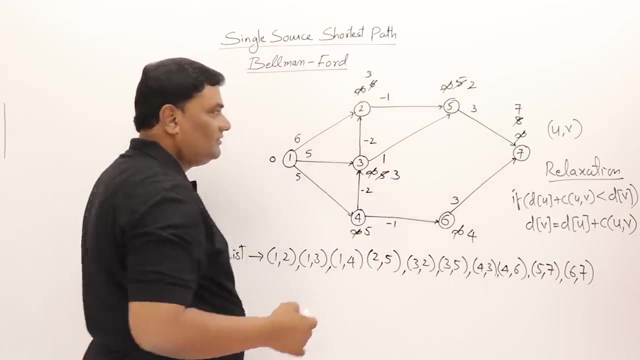 so don't change that one. 1 comma 3: 0 plus 5, 5, that is 3. don't change that one: 1 comma 4: 0 plus 5, only no change then 2 to 5: 2 to 5, so 3 minus 1, 2, this is 2. that is changing again. so 3 to 2, so 3 is. 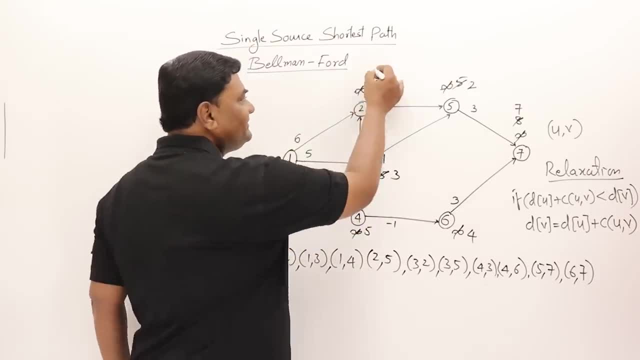 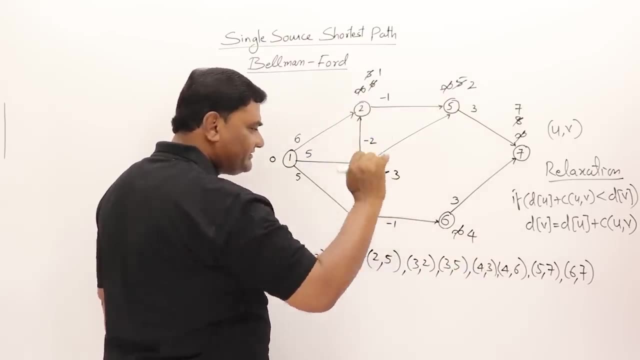 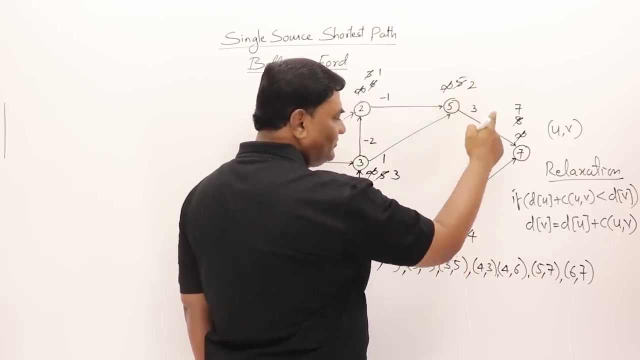 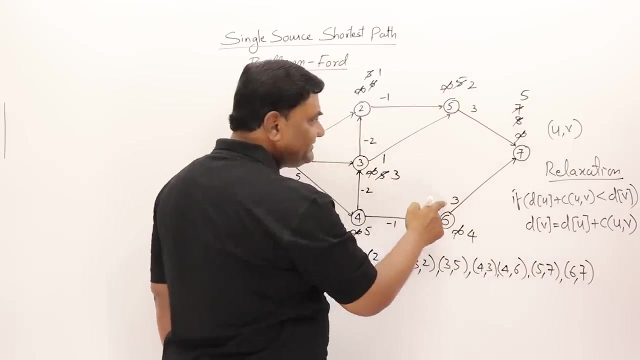 how much: 3, 3 minus 2 is 1, so this will change 1. then 4 comma 3, 4 comma 3: 5 minus 2, this is 3, this is 0, and 2 plus 3, 5 this is 7. so change it to 5. then 6 comma 7: 4 plus 3 is 7 and it is 5, no change. 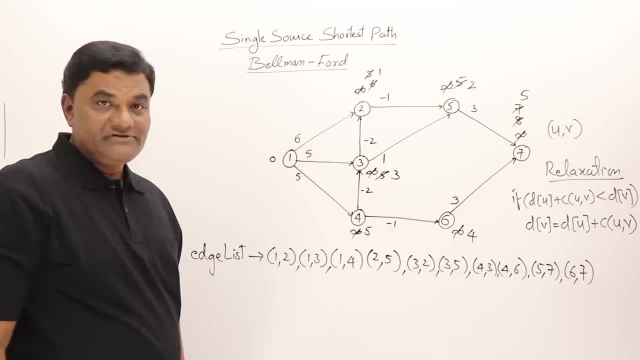 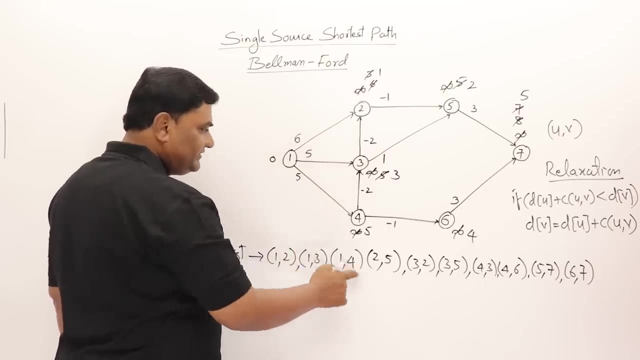 let it be as it is. i have completed two times. four more times i have to do 1 comma 2. this will not change 1 comma 3. this will not change 1 comma 4 also will not change. then 2 comma 5: 1 minus 1. this. 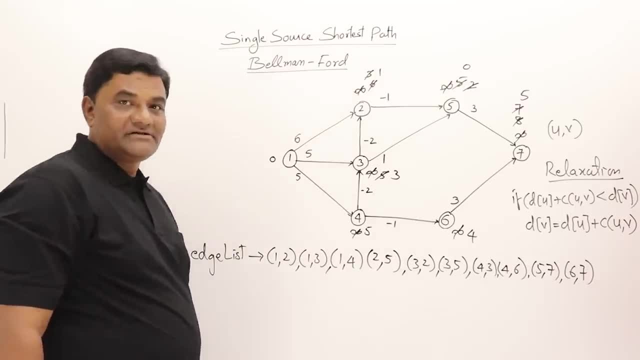 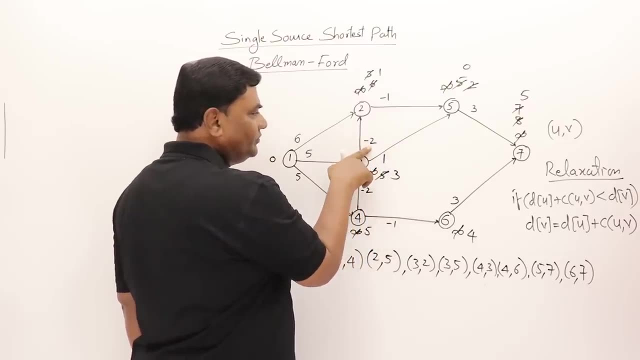 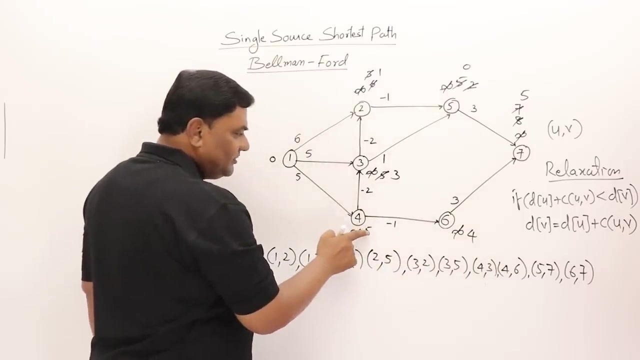 becomes 0, this becomes 0, right. then 3 comma 2. so 3 is how much? 3? 3 minus 2. 3 minus 2 is 1, already 1. now no more changes. then 3 to 5. so this is 3 plus 1. 4 already it is 0, that is better. 4 to 3. 4 to 3 is how much? 5 minus? 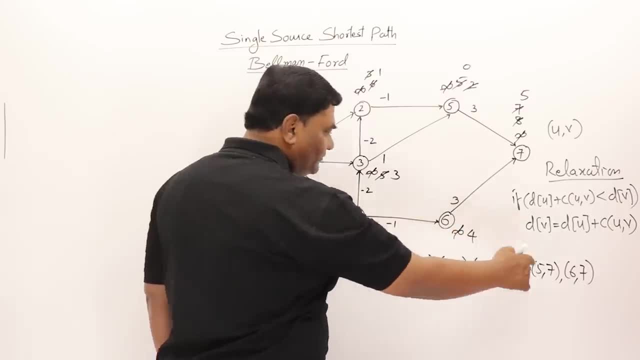 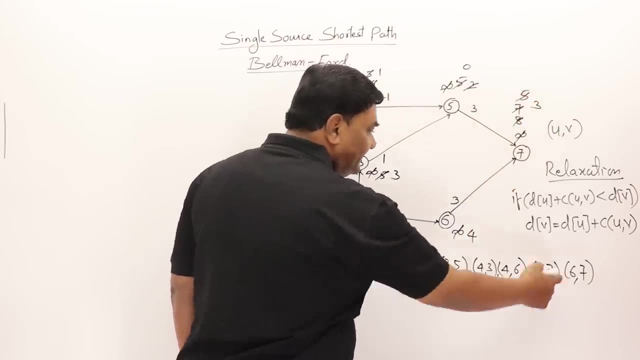 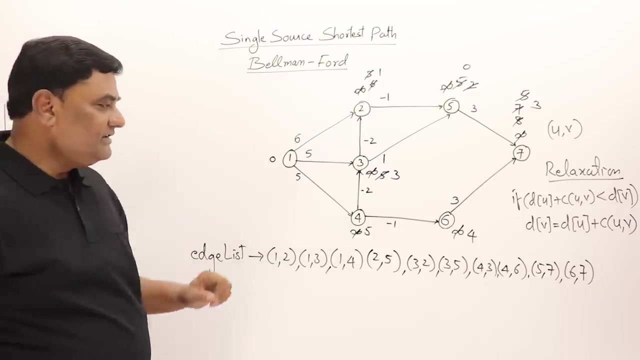 2, that is 3, no change. 4 to 6: 4, no change. 5 to 7. 5 is how much? 0, 0 plus 3, 3, this becomes 3, then 6 to 7, 4 plus 3, 7. that 3 is better right. so i am updating there only, so three times i have. 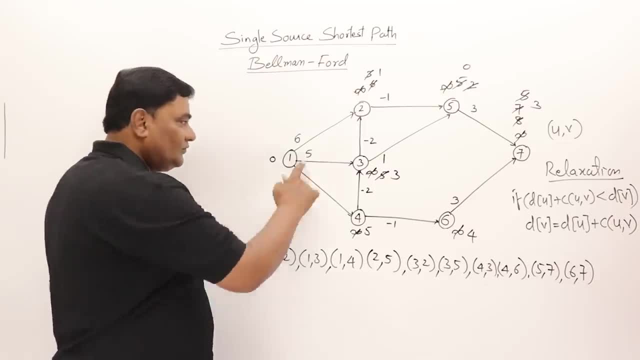 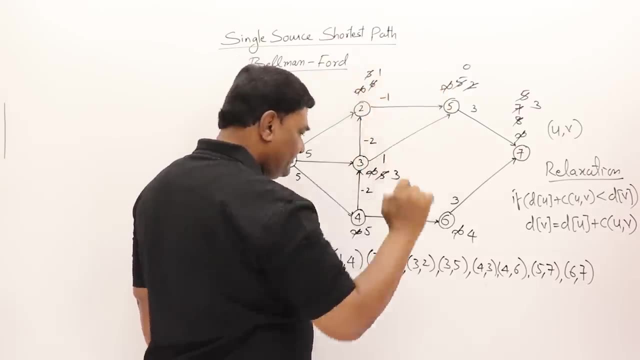 completed three more times i have to do. 1 to 2 will not change. 1 to 3 will not change. 1 to 4 will not change. 2 to 5, 2 is how much 1, 1 minus 1, 0. that is not changing. then 3 to 2. so 3 to 2, 3 is. 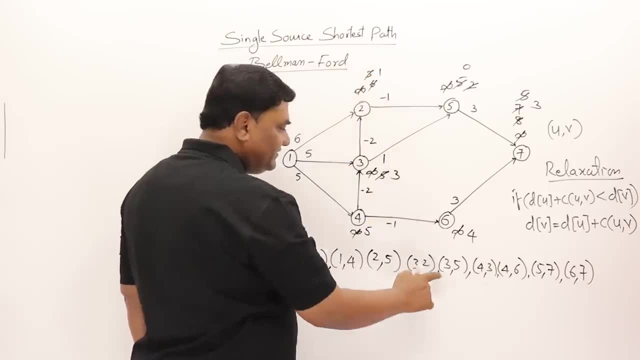 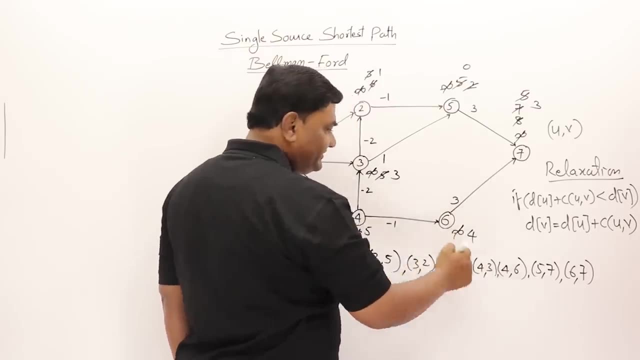 how much? 3 minus 2, 1, 1, it's already 1. then 3 to 5. so this 3 plus 1, that is not changing 1 to 4, that is better. 0, 4 to 3 will not change. 4 to 6 will not change, then 5 to 7: 0 plus 3, 3 only. 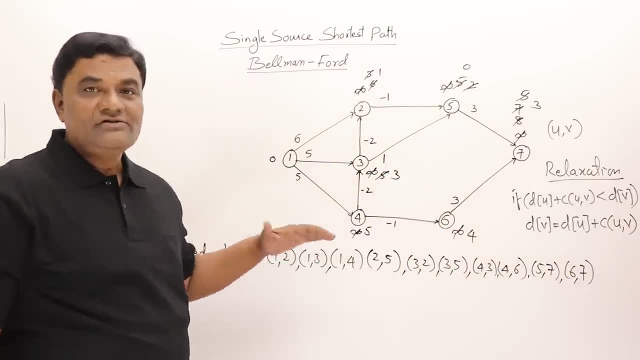 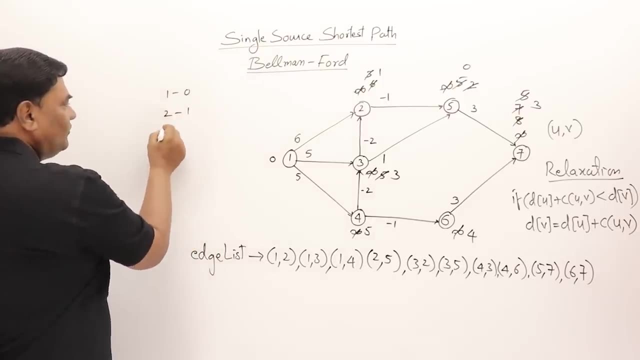 6 to 7: no change. now this has stopped changing. so what are the results i got? what x1 is 0, what x2 is 1, what x3 is 3, what x4 distance is 5, what x5 distance is 0, what x6 distance is 4, what x7. 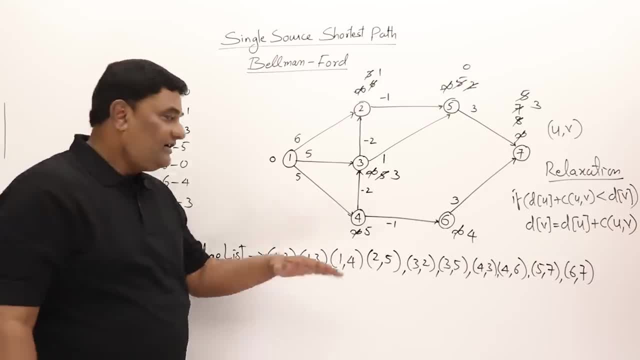 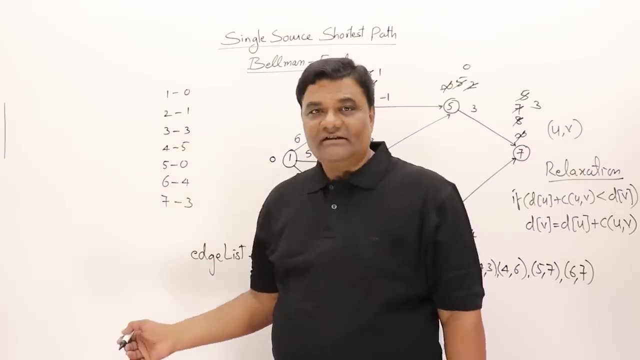 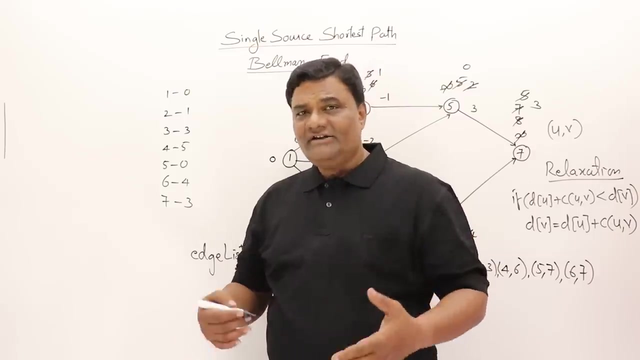 distance is 3. these are the distances i got. if i continue for two more times also, i'll get the same result. so finally, these are the shortest paths. you can observe that. so, as i am doing it manually, i have stopped. but when you write in any algorithm for doing the same thing, it will continue for n minus one time. 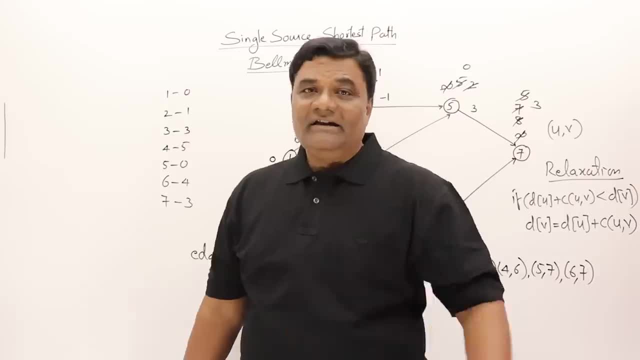 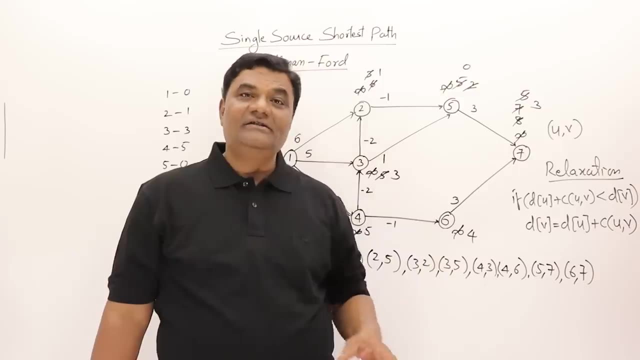 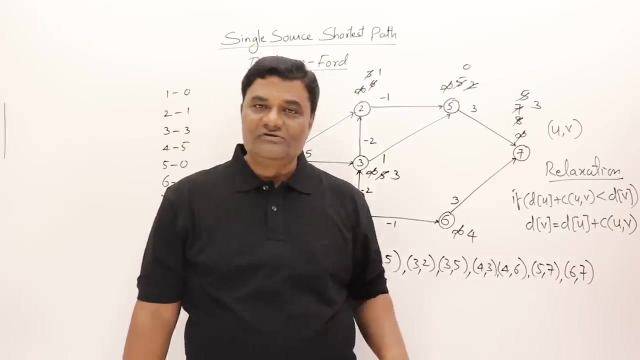 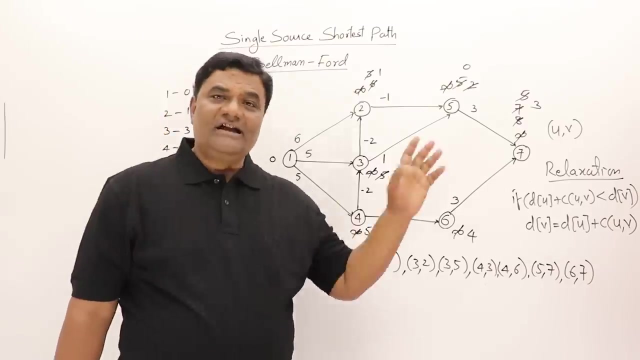 and some graphs may get the shortest path in just one time relaxation only, and some graph may relax completely, get the shortest path in the last relaxation. so in this graph we find that after the third one onwards, there are no change, no more changes. i have taken the shortest paths. so this is how bellman ford algorithm works. let us get the time complexity. 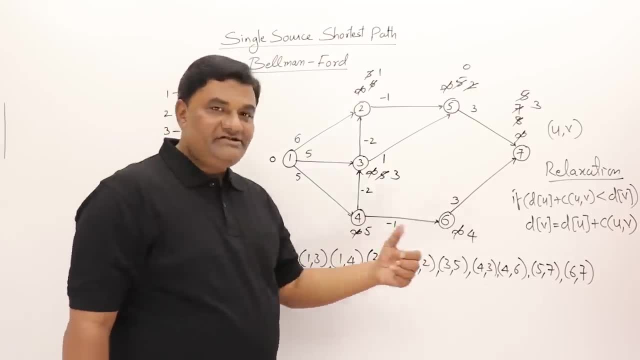 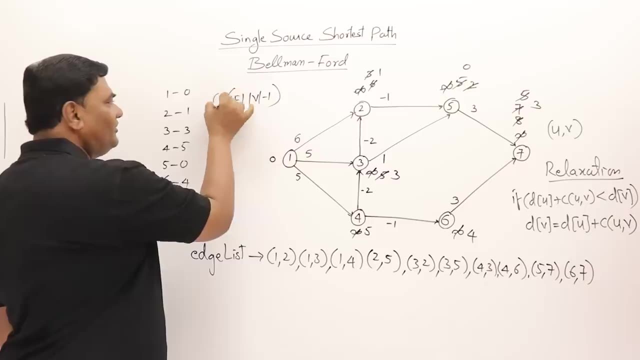 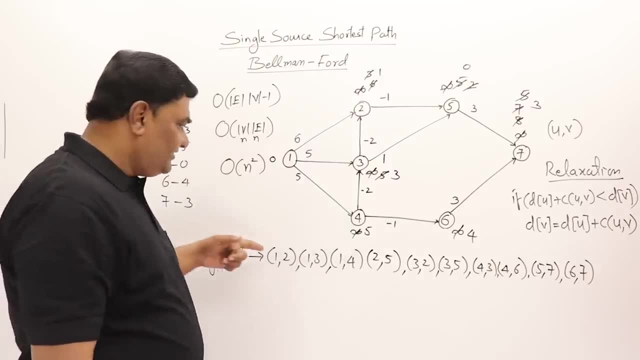 square n, so it depends on the number of edges. if this is a complete graph, then how many edges will be there in a complete graph? a complete graph means there is an edge between every pair of vertex. so total, how many edges will be there? n into n minus one by two edges will be there. 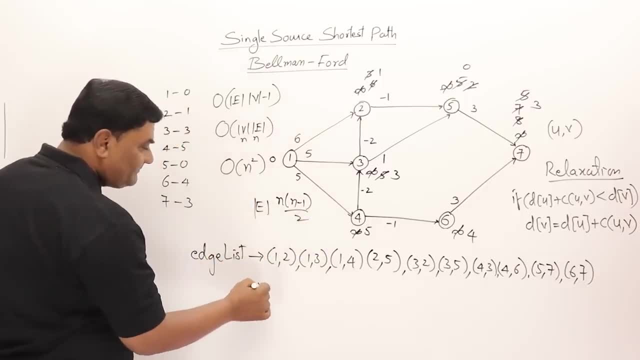 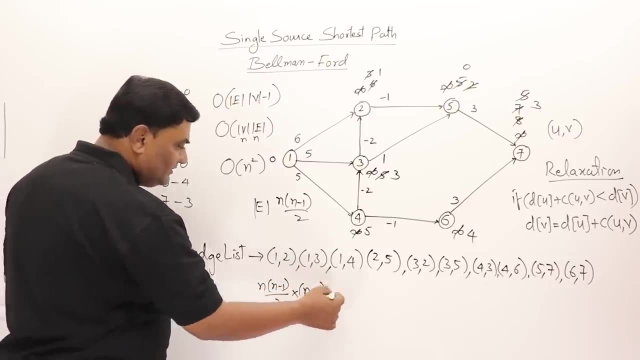 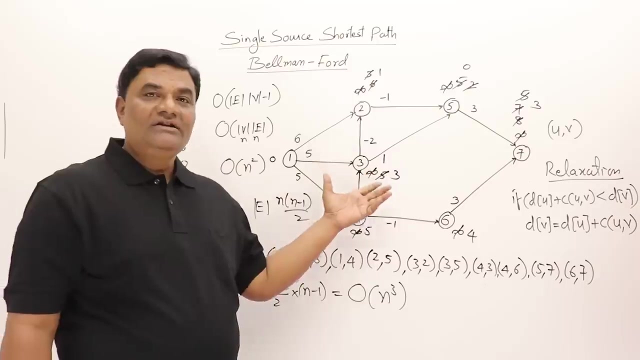 so if these many edges are there, then the time will be n into n minus one by two into number of vertices minus one, n minus one. so if you simplify this one, this will be order of n cube. so in case of complete graph, bellman ford algorithm may take even n cube time right. otherwise minimum time we say it takes n square. 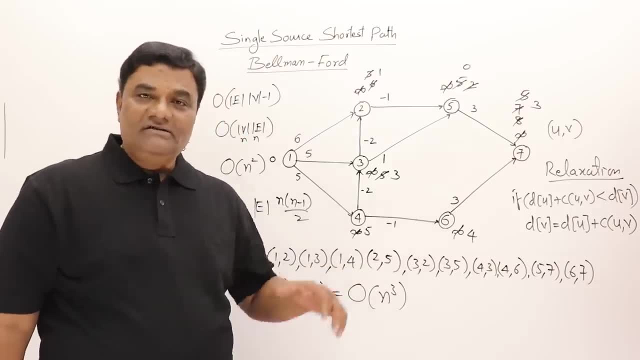 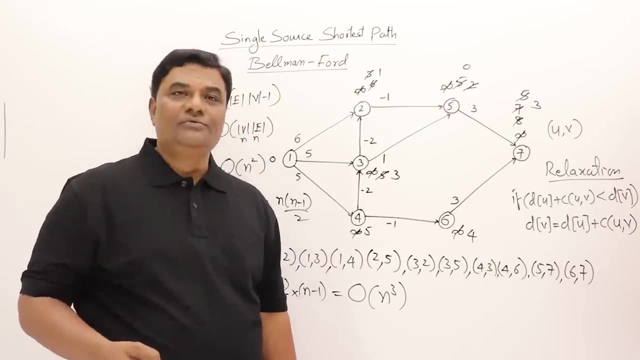 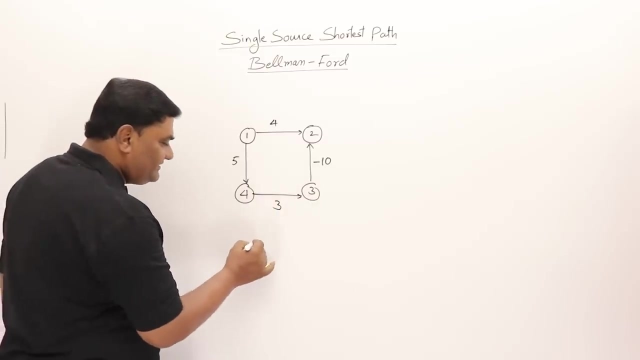 and at most it may take n cube time, that is if the graph is complete graph. now i will take a small example and solve it and also i will show you drawback of bellman ford. a small example. i will take the list of edges first of all. i will take the edges. 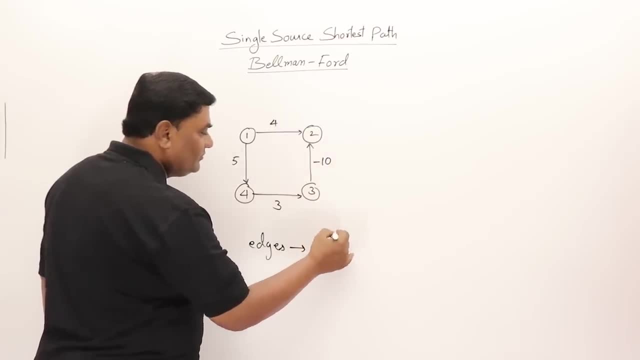 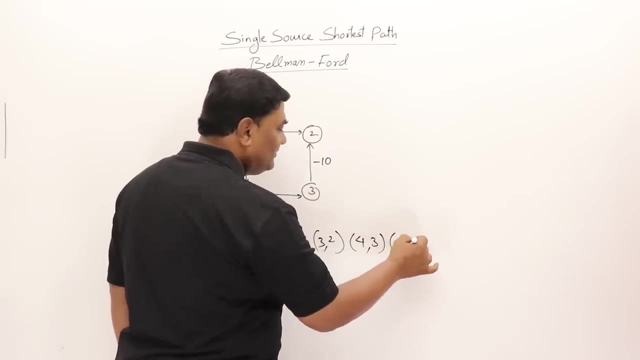 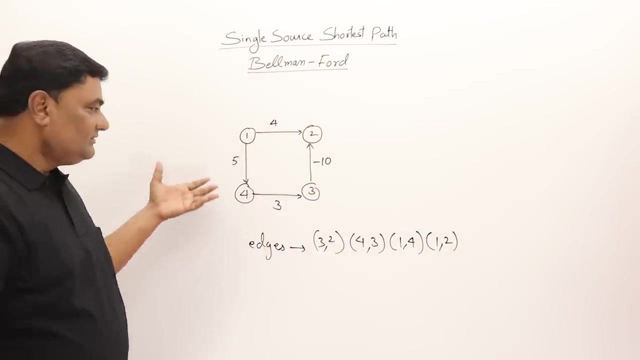 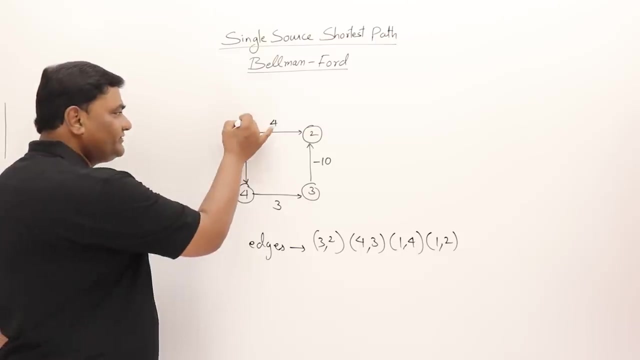 starting from here, first i will take three comma two, then i will take four comma three, then one two four, then one two two. see, just to make you feel how the relaxation are done. i have taken the vertices in reverse. i should have started from vertex one. now let's solve this. my source vertex is zero and mark all of them as infinity mark. 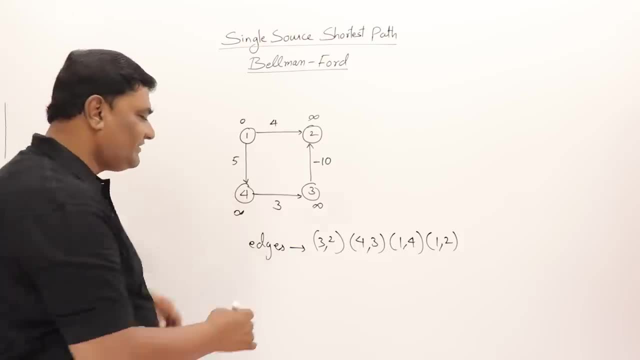 all of them as infinity. how many times i should relax? there are four vertices, so i should relax that for four minus one. that is three times. so let us relax all the edges one by one. first, three comma: two: infinity minus ten is infinity only. so that is no change, it is. 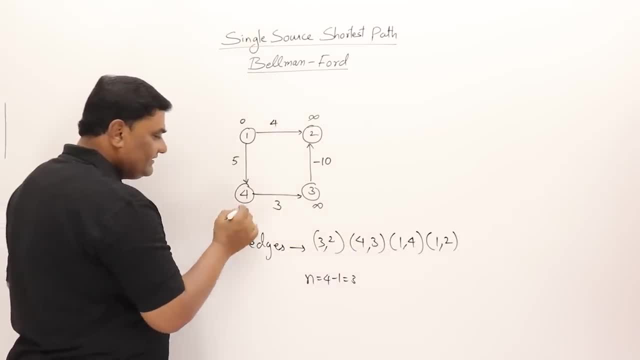 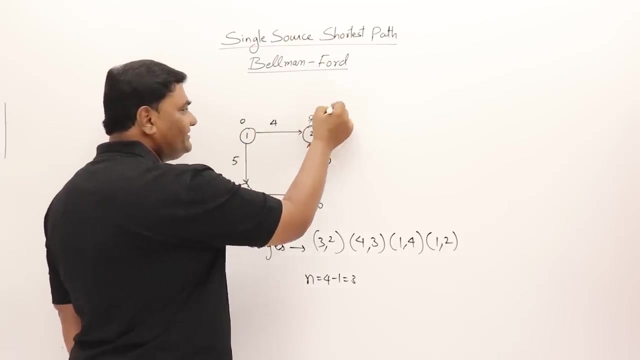 already infinity. four comma three. infinity plus three is infinity only. and this is already infinity. then one comma four. one comma four. zero plus five. five is less than infinity, so change it to five. then one comma two. zero plus four. four is less than infinity. change it to four one time i. 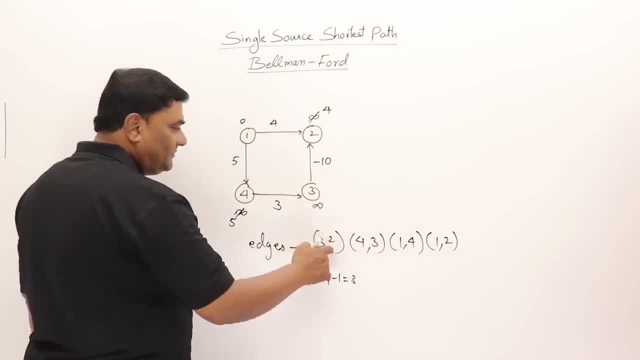 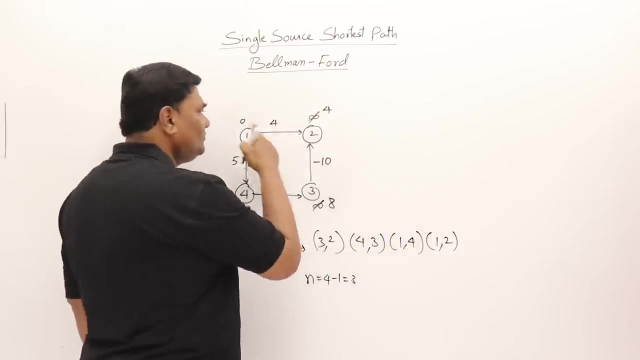 already have relaxed second time. three comma two, infinity minus ten as four, that is better. four comma three, five plus three is eight. this is better than infinity. so make it infinity. one, two, four, 0 plus 5, 5 only. 1 to 2, 0 plus 4, 4 only. 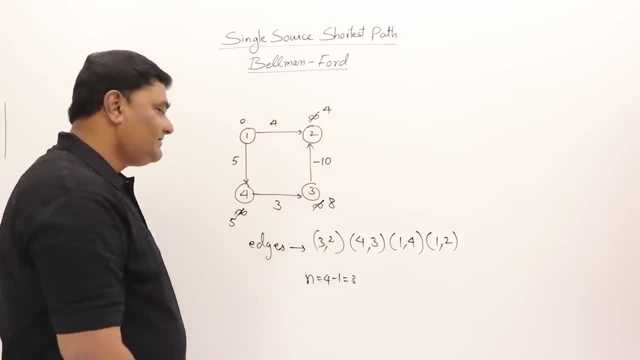 Two times I have completed. One more time I have to complete. Let us check 3 to 2,. 8 minus 10 is minus 2.. Minus 2 is smaller than 4.. Now you can see that I got. 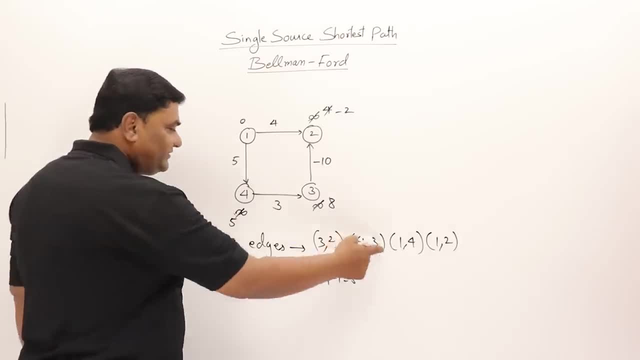 the correct answer for vertex 2. now Then 4 to 3, 5 plus 3, 8, only 1 to 4, 0 plus 5, 5, only 1 to 2, 0 plus 4.. And that is not greater, not less. 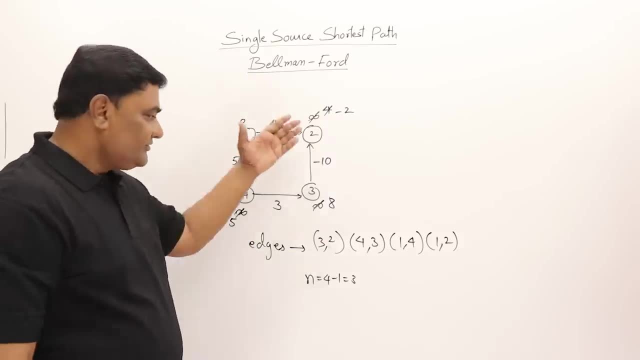 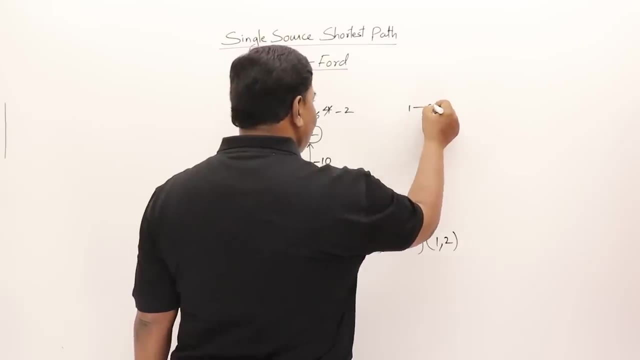 than minus 2.. So minus 2 is better. Let it be as it is. So I have relaxed them for 3 times and I got the shortest paths. So what are the shortest paths? Vertex 1 is 0.. Vertex 2 is: 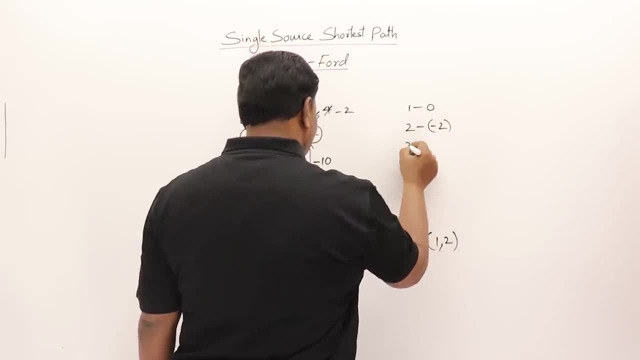 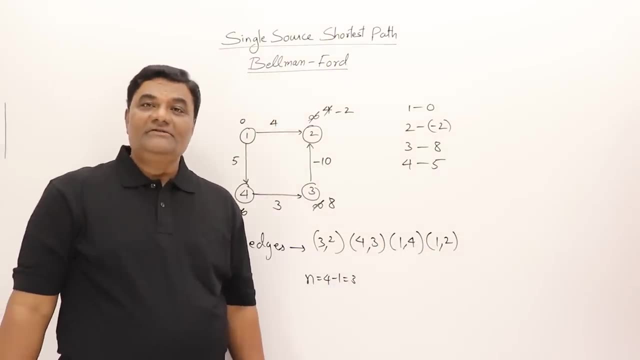 minus 2.. And vertex 3 is 8.. Vertex 4 is 5.. These are the shortest paths for starting vertex as 2.. So Bellman-Ford has got the answer, even when there are negative edges. So this is the. 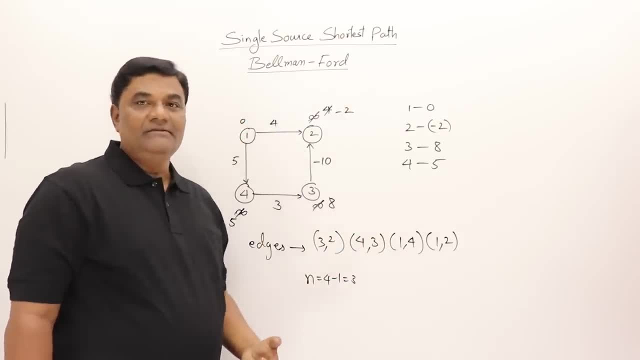 answer: If I relax this for one more time and see, let us what happens: 3 comma 2, 8 minus 10 minus 2, only 4 comma 3, 5 plus 3, 8, only 1 to 4 and 1 to 2, all are same. So if I relax one more time, 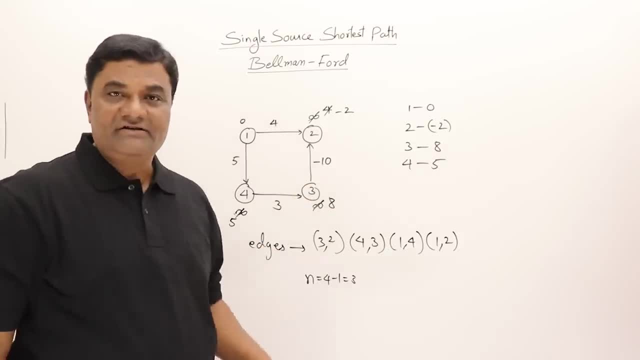 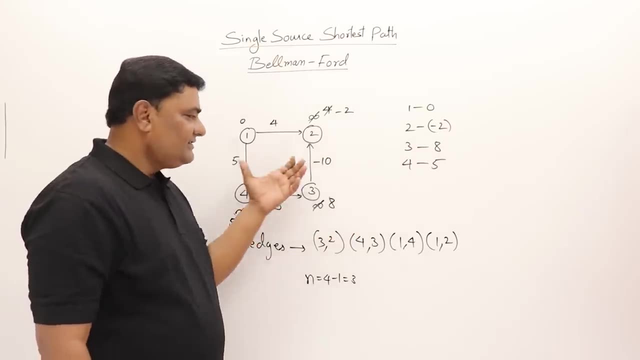 extra. also, there is no change. That means the answers are perfect. Now let us see the drawback of Bellman-Ford. I will take the same graph, only but a small change: The same graph. I will add one more edge, that is 2 to 4, and I will make it as 5.. 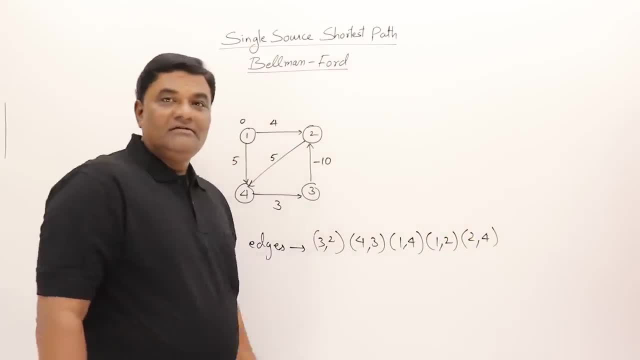 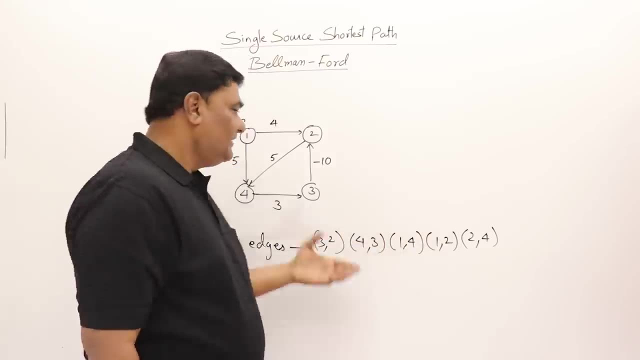 So this is 2 to 4.. Now let us relax them. I have to relax them for 3 times So quickly. I will do it, because already till here I was doing it. Let us do So: 0, infinity, infinity and infinity. 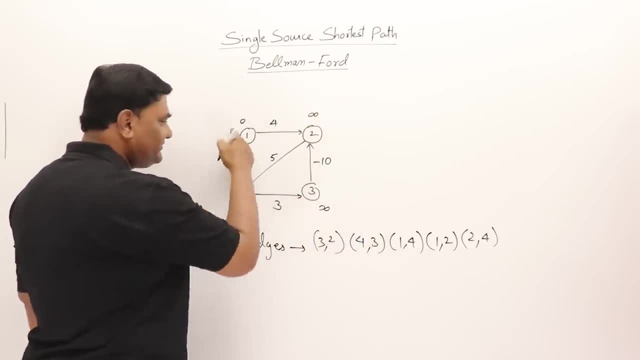 3 to 2,. infinity only 4 to 3,. infinity only 1 to 4,. 0 plus 5, this is 5.. 1 to 2 is 0 plus 4,, this is 4.. 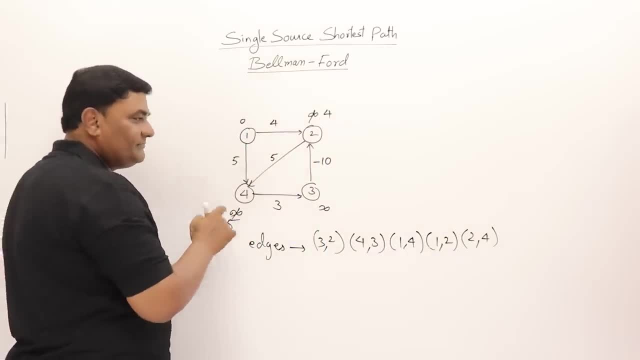 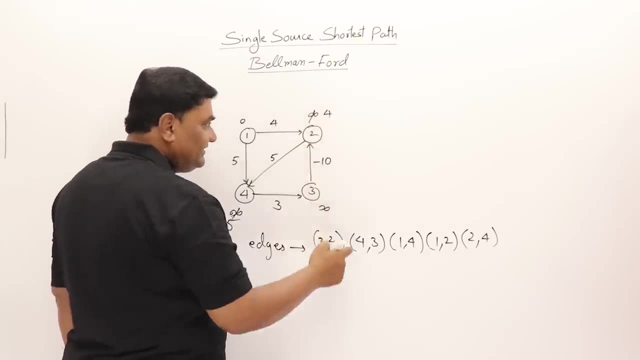 Now 2 to 4, 0 plus 5, this is 5.. 1 to 2 is 0 plus 4, this is 5.. 4 plus 5, 9, this 5 is better, No need of changing One time over. Now 3 to 2, infinity minus 10, that is infinity. 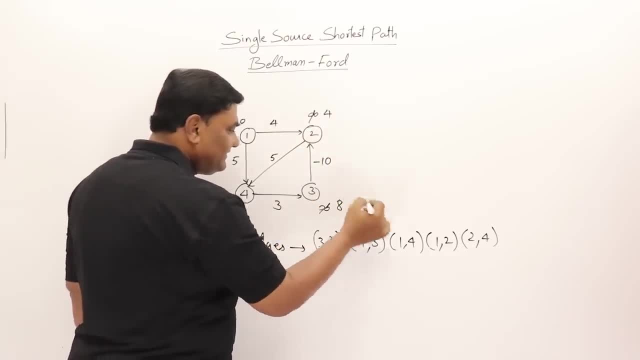 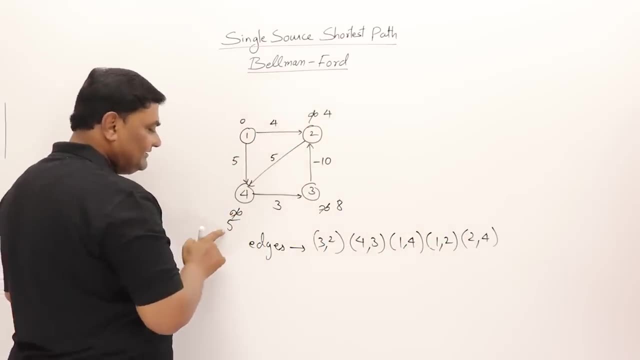 So 4 is better. 4 comma 3, 5 plus 3, this is 8.. Then 1 to 4 is same thing, only. 1 to 2 is same thing, only Then 2 to 4, 4 plus 5 is 9 and this is 5, that is better. 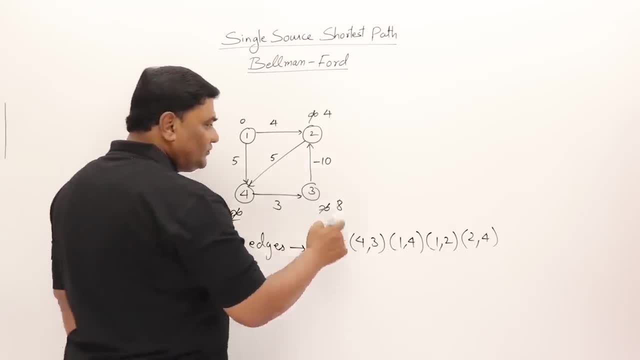 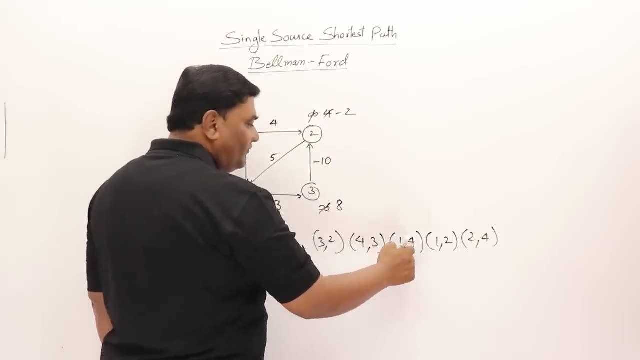 2 times completed. The third time: 3 to 2,, 8 minus 10, minus 2.. Then 4 to 3,, 5 plus 3, is 8.. 8 is there. 1 to 4, is 5 only. 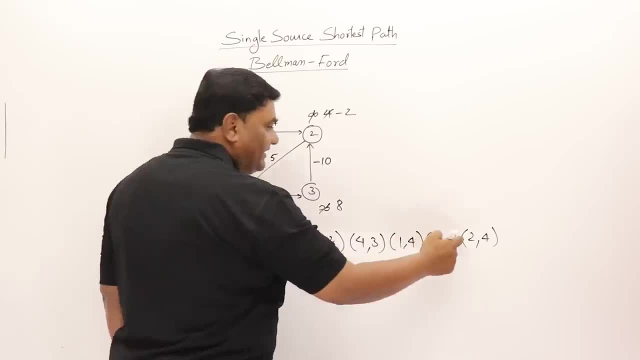 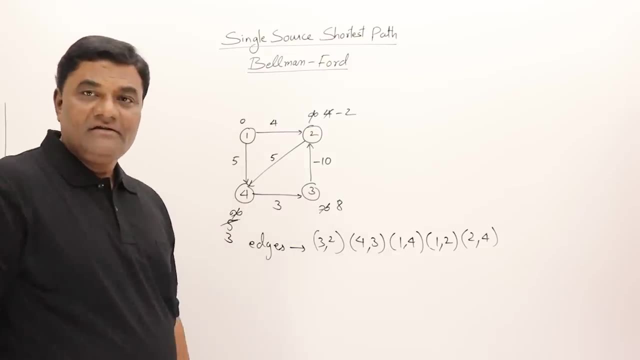 1 to 2,, 0 plus 4, so minus 2 is better. Then 2 to 4, minus 2 and 5 is 3.. This 4 is changing Right. So this was the third time I have done and I got this answer. 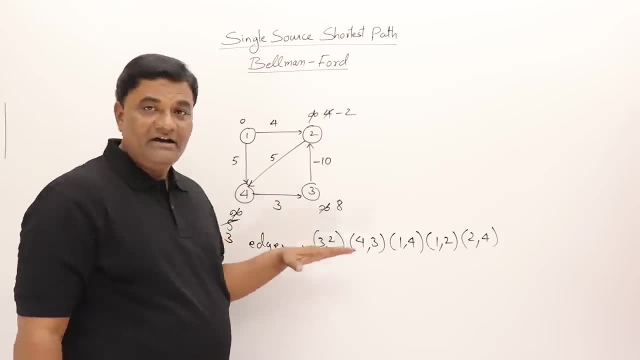 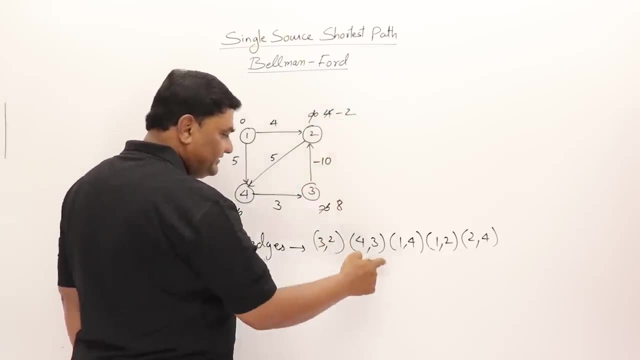 Let me try for one more time. Already n minus 1 time I have done, But let me try one more time and check: 1 comma 2, 8 minus 10 is minus 2, only. Yes, 4 comma 3, 3 plus 3, 6.. 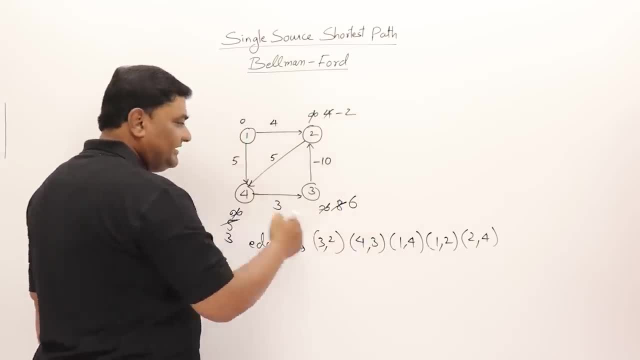 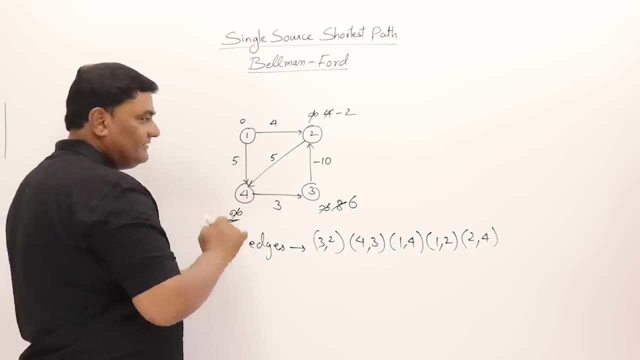 Oh, this is changing. 1 to 4 will remain same. 1 to 2 also remain minus 2 only And 2 to 4, minus 2 to 5 is 3 only. Minus 2 plus 5 is 3 only. 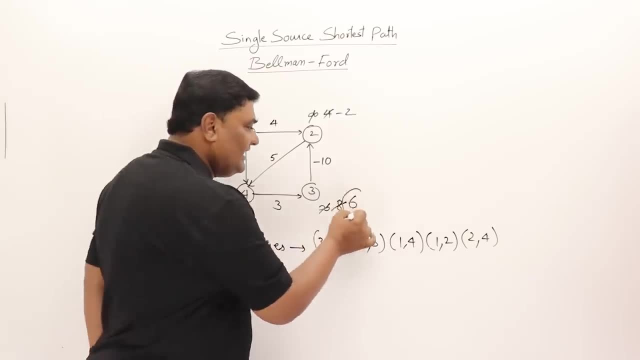 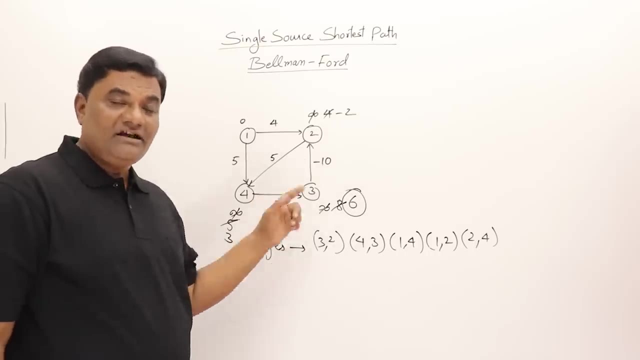 So one more vertex has just now relaxed. That should not happen After completing for n minus 1 time. I should get the answer. If I repeat it for one more time, if I relax all the edges, there should not be any change at all. 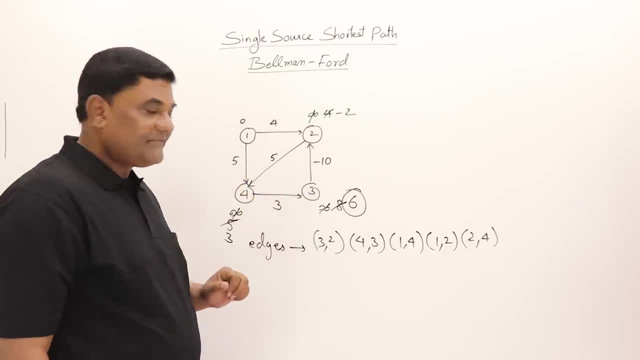 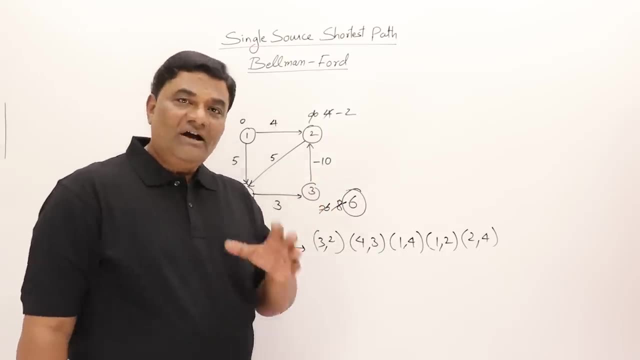 If I do one more time again, something will change, See 3 comma 2, 6 minus 10, minus 4.. So that's what there is a problem. So why we got this problem? Bellman-Ford is unable to solve this one. 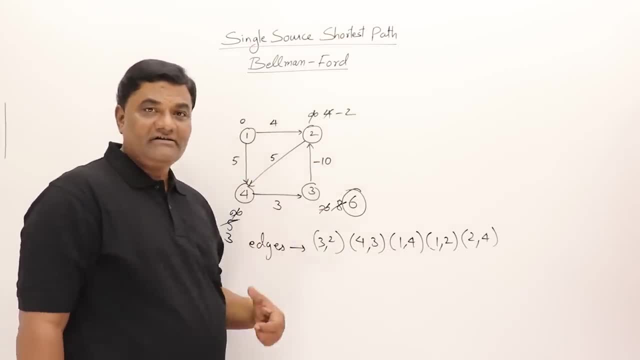 After performing for n minus 1 time. also, I am not getting the correct answer. Still they are getting relaxed. So even if I do it without Bellman-Ford directly, if I try to do, I cannot solve it. Reason is: 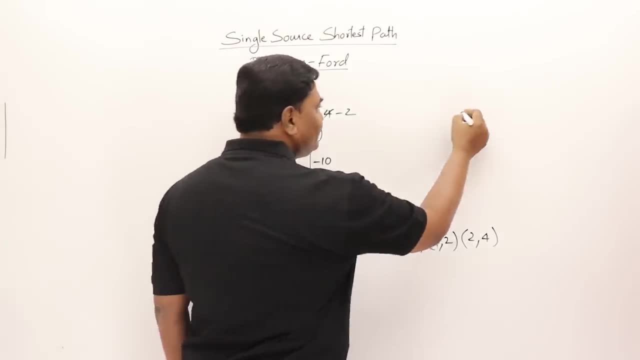 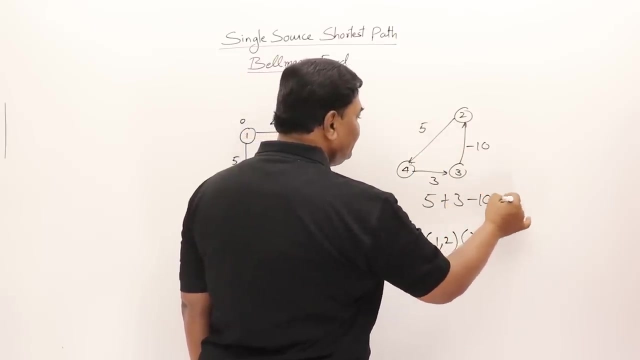 there is a cycle of edges that is 2 and 4 and 3.. So this is forming a cycle. This is minus 10 and 3 and 5.. So if I add this, 5 plus 3, 8 minus 10 is minus 2.. 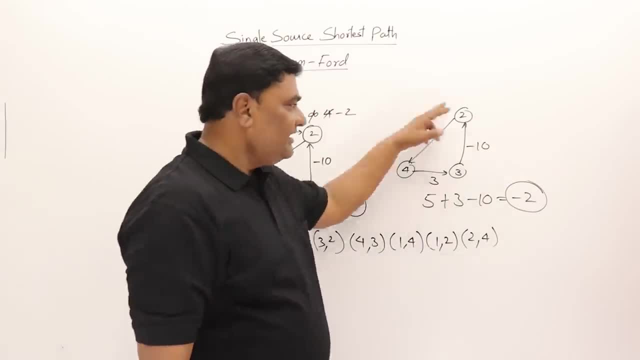 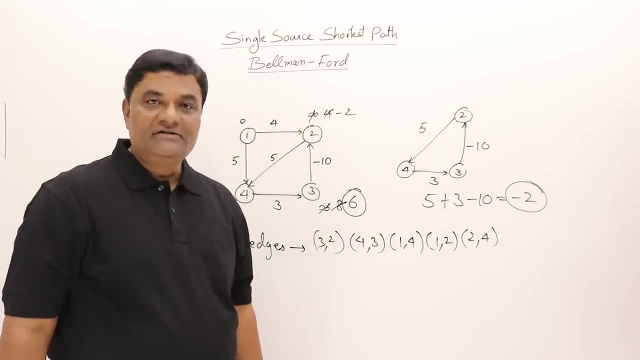 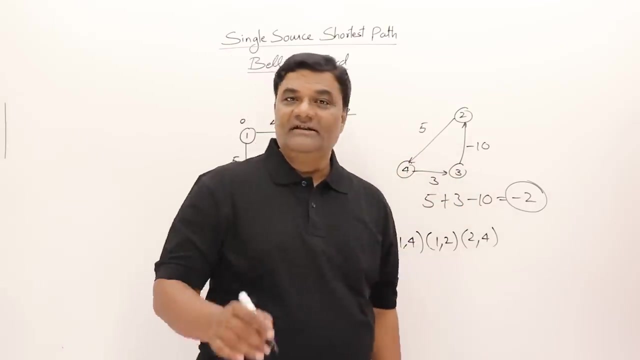 The total weight of a cycle is negative. So in this way I will be going on getting the path reduced every time, So there is no end of this one. So I cannot decide or freeze the answer. So if there is a negative weight cycle, then graph cannot be solved.